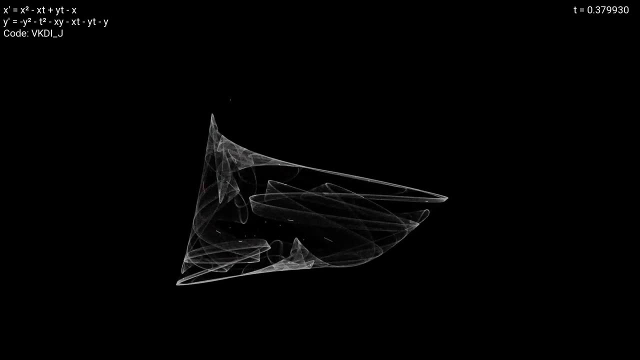 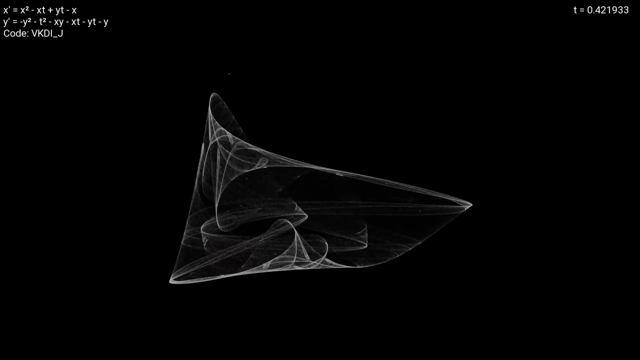 This mathematical art is an example of what I call chaos equations. As I was going through my old game maker projects, I remembered I used to make a bunch of these with it, and they were so cool and so simple. I decided to make a new, polished version. 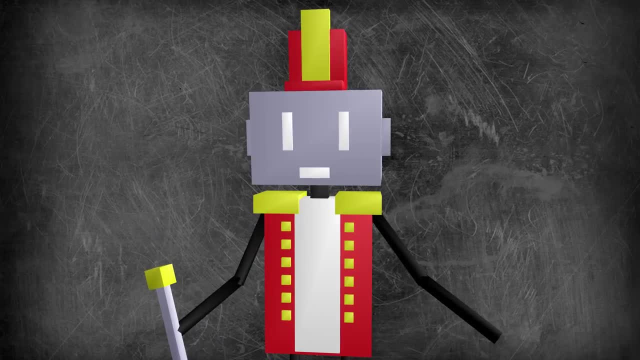 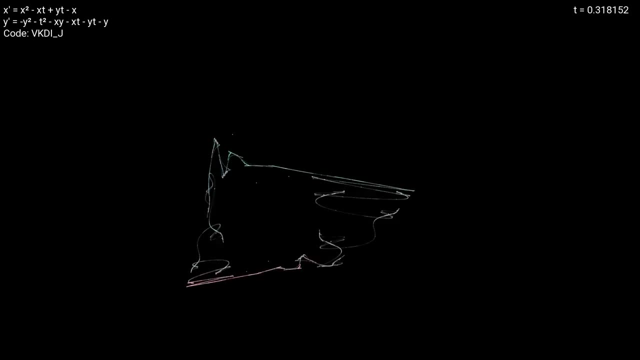 And I do really mean simple. You don't need more than middle school math to understand it. no imaginary numbers or anything complicated. These are dynamic systems, which means they change over time. Time is represented by the variable t. It starts at a low value and then slowly increases as the animation progresses. 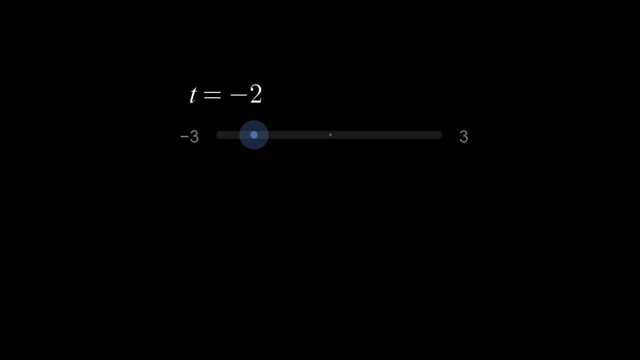 At every time step we start with a point whose coordinates are initialized to t. Then we apply an equation to update the point. It can be any equation. I just use random ones in the program and, surprisingly, most of them actually look good. 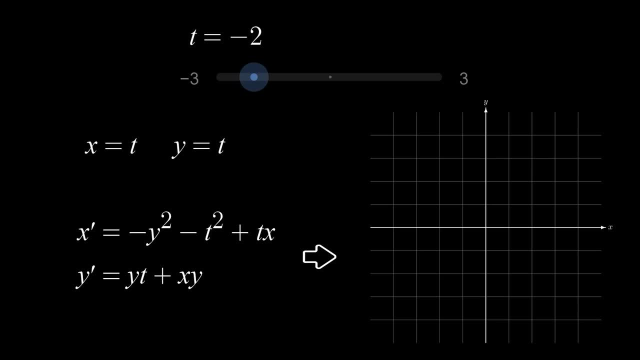 Anyway, once we have the new point, we draw it to the screen with a unique color and then repeat. So, for example, we draw this point in green, then apply the same equation again to update the point, Maybe draw this second one in blue, Apply again, draw this one in red and repeat. And as time changes, those points change as well. 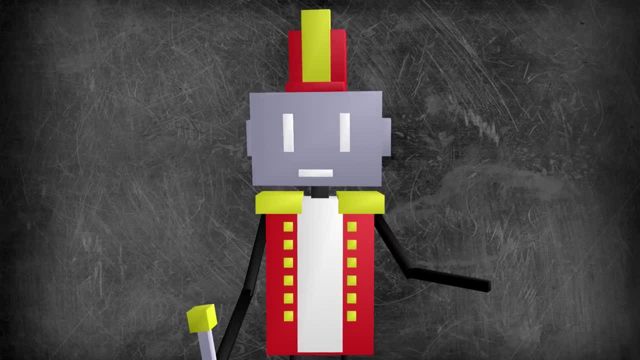 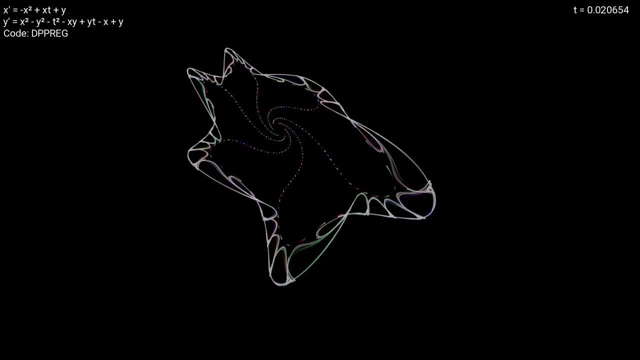 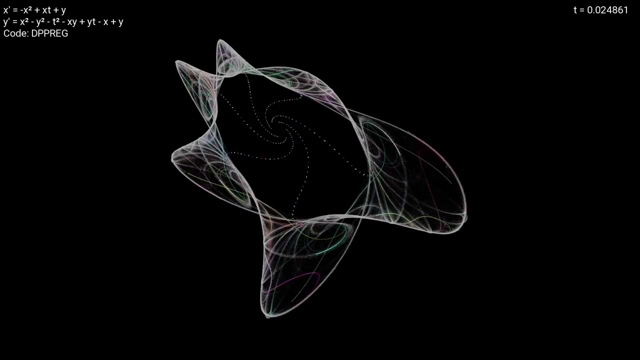 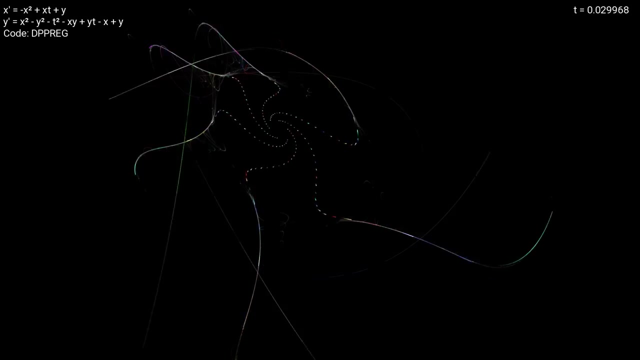 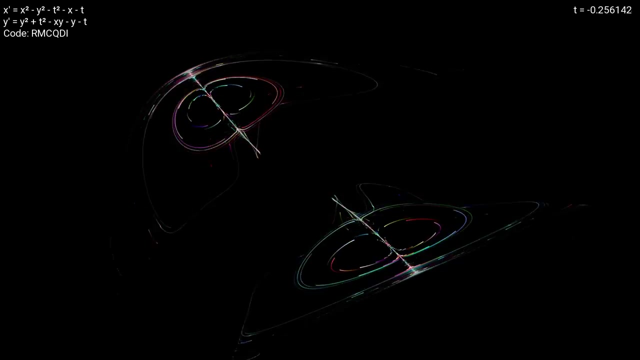 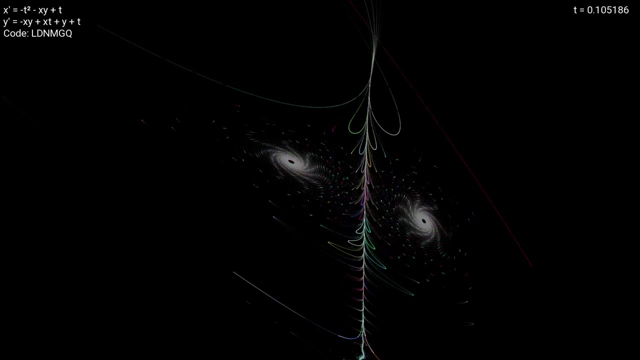 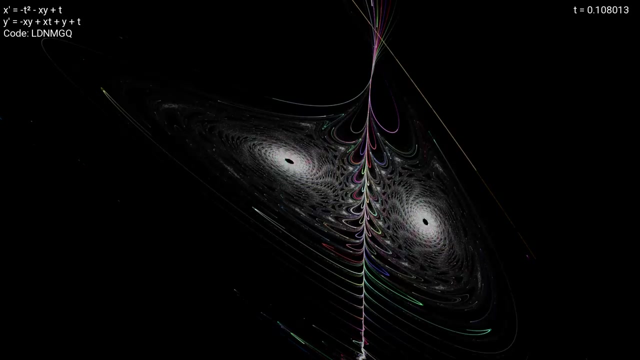 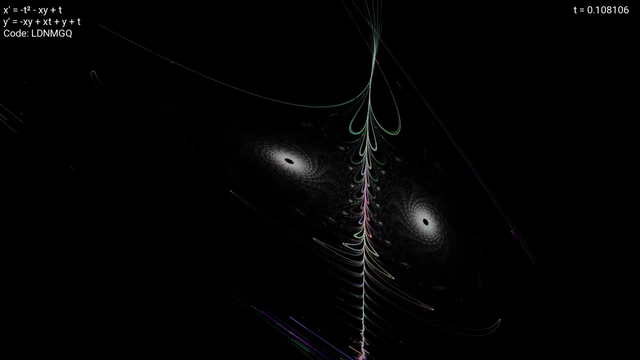 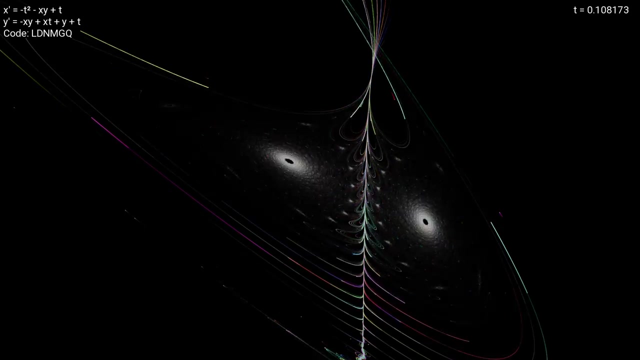 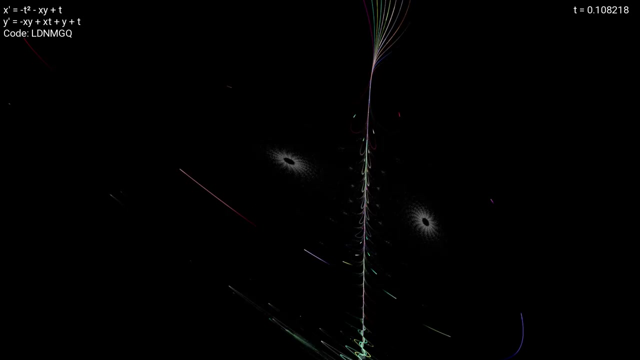 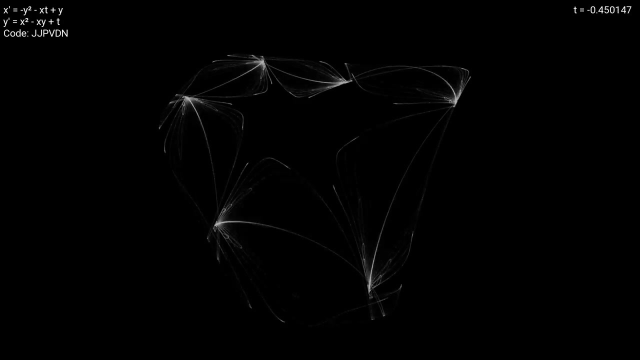 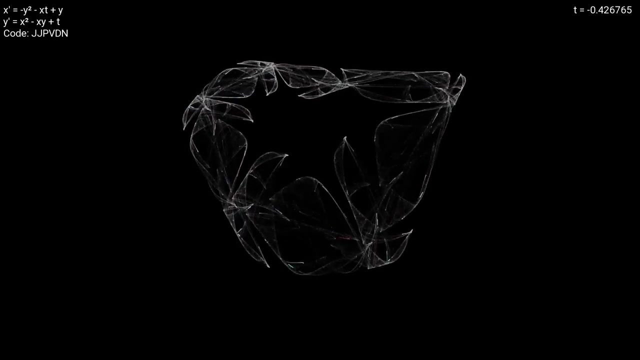 That's literally it. I just added some fancy trails and tried to dynamically change the speed, so it speeds up when nothing interesting is happening. Here are some of my favorites so far. See you in the next video, Thank you, Thank you. 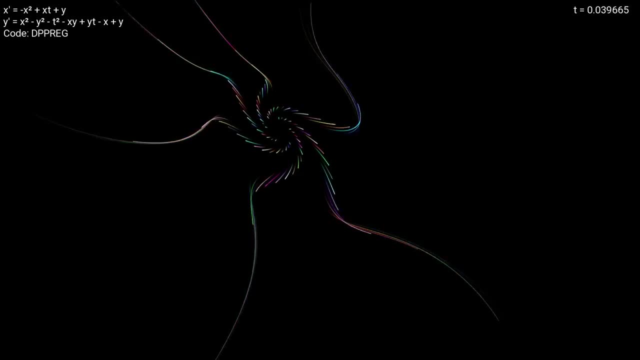 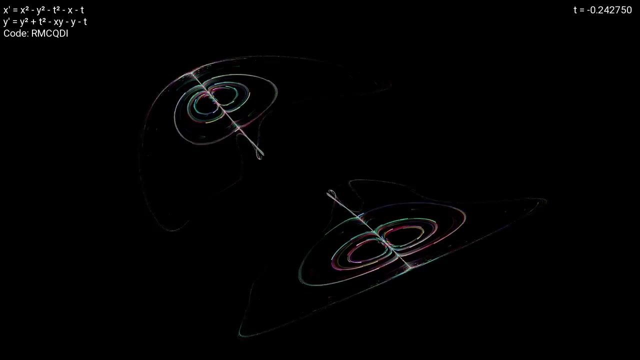 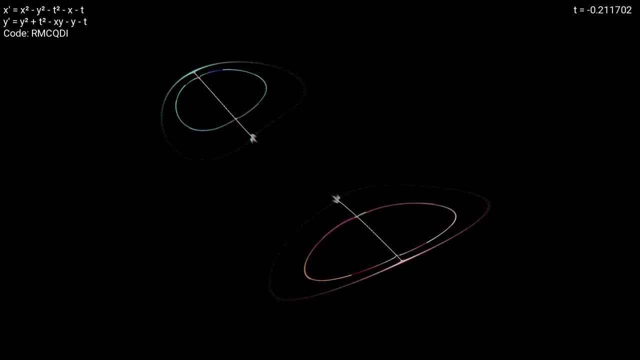 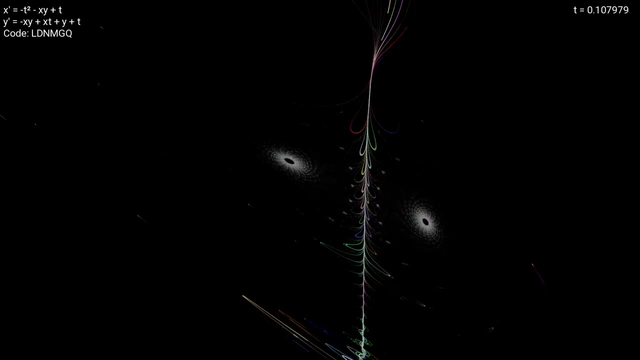 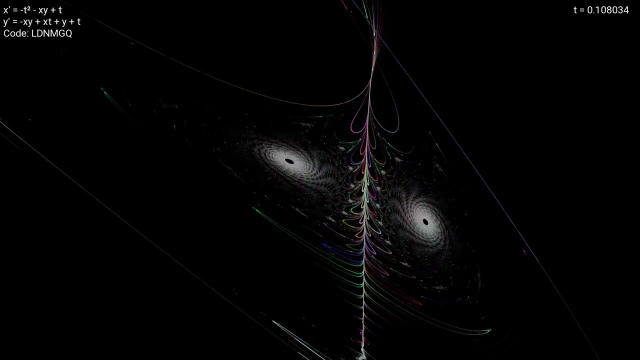 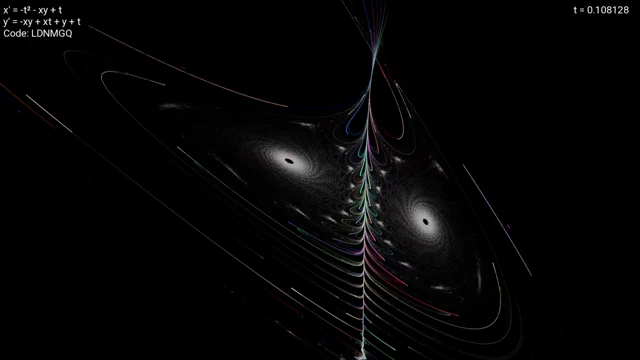 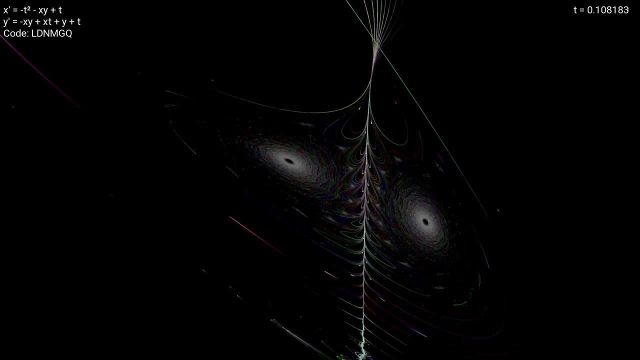 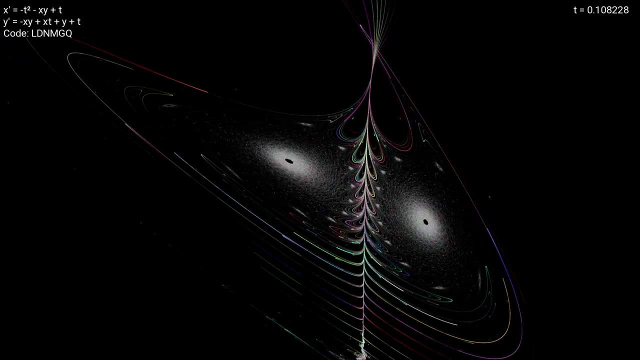 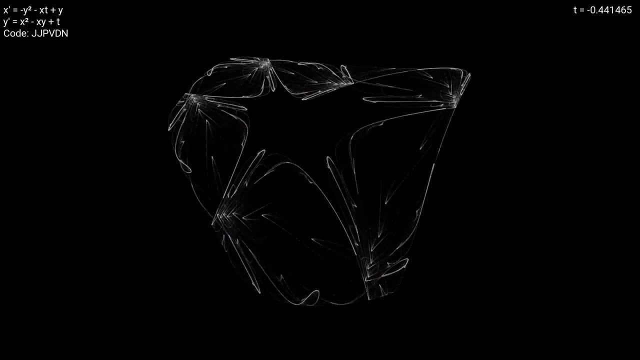 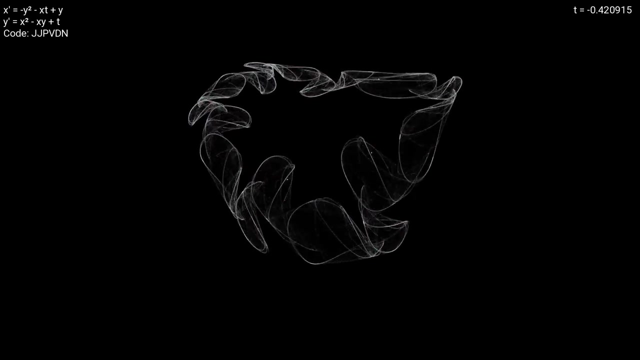 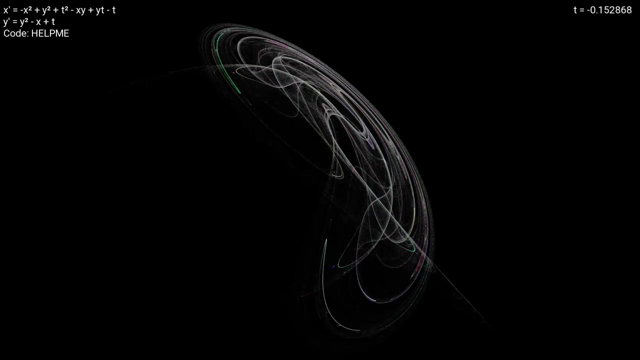 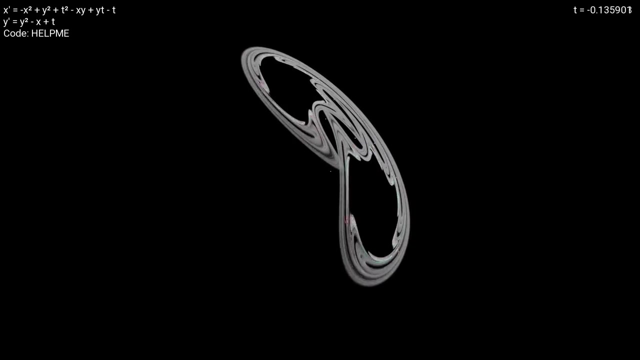 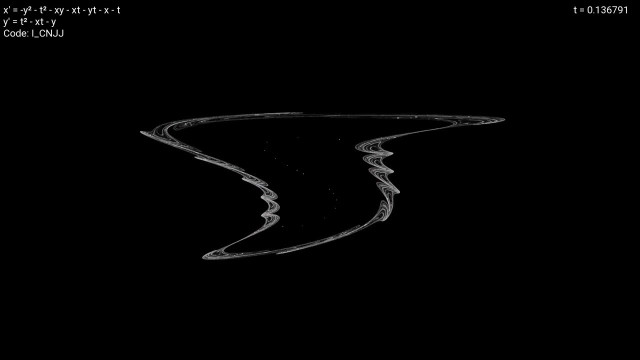 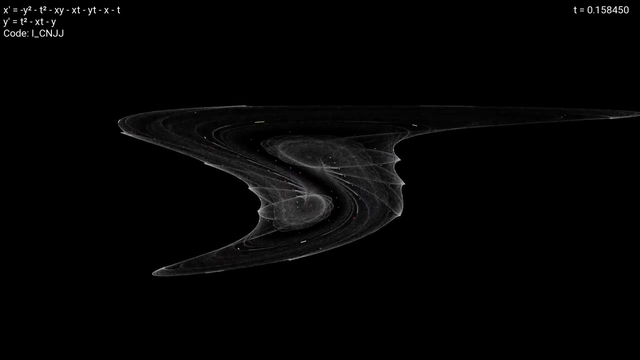 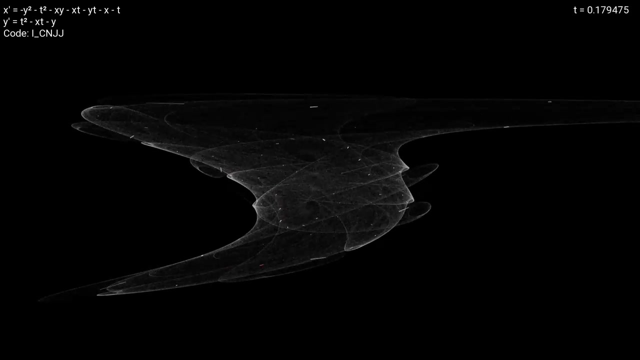 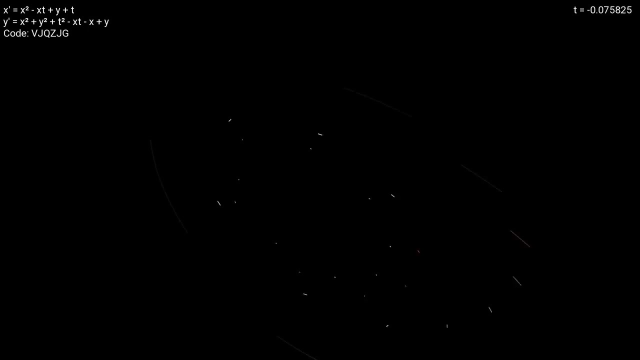 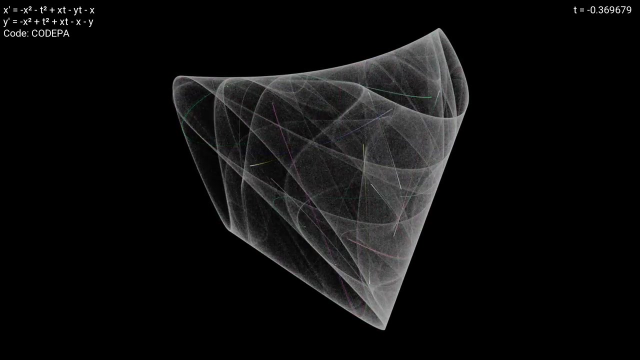 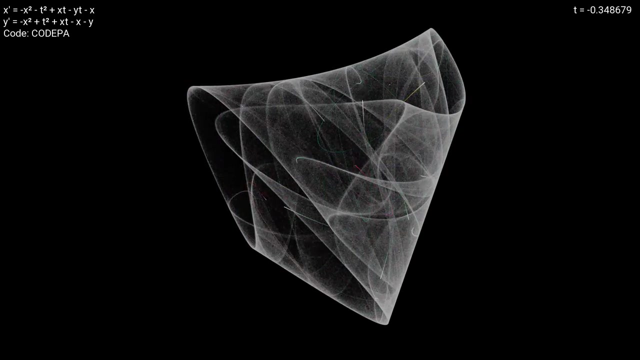 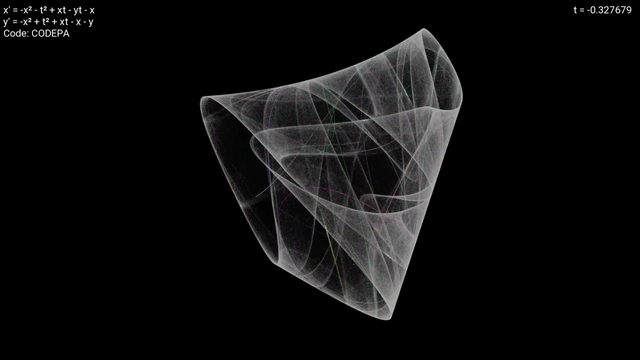 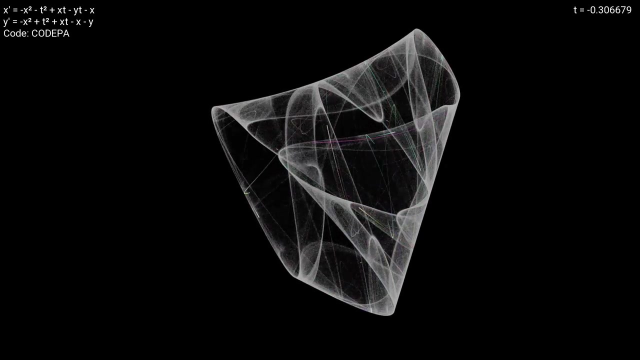 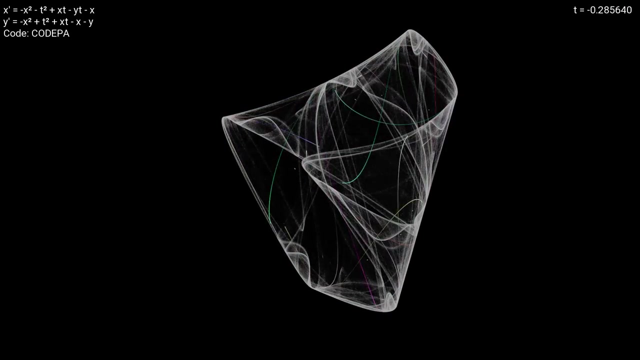 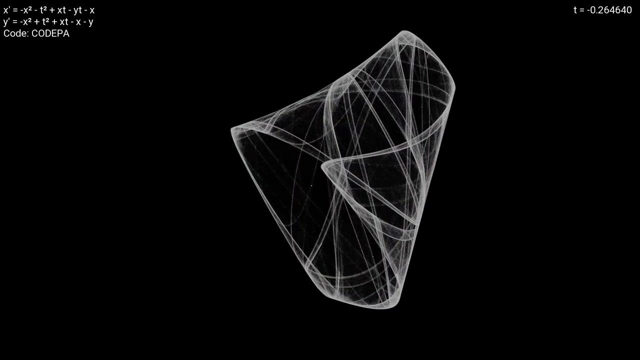 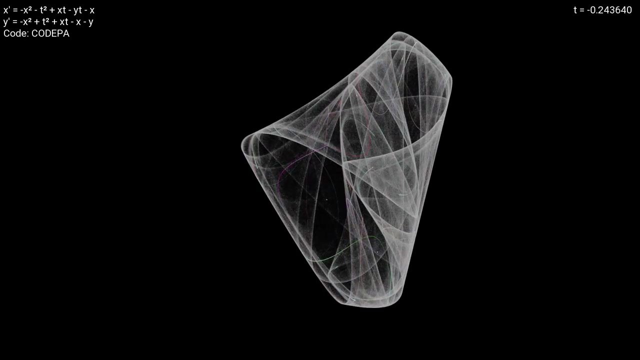 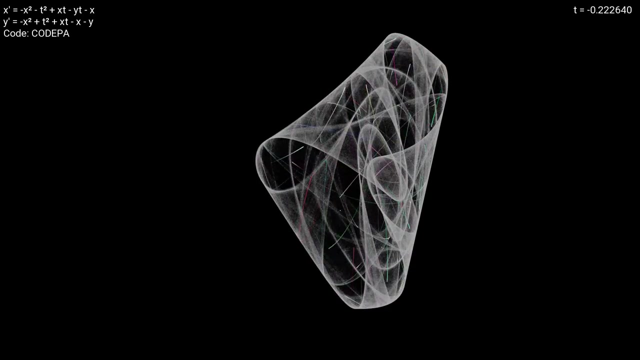 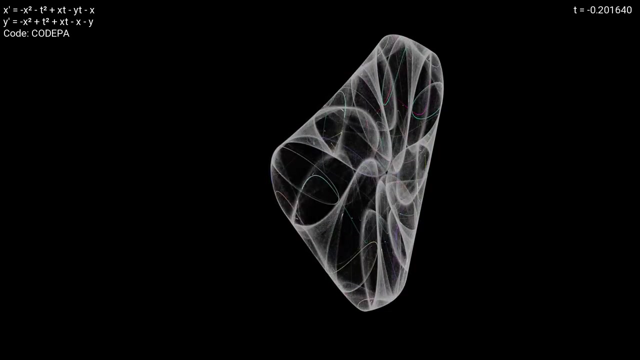 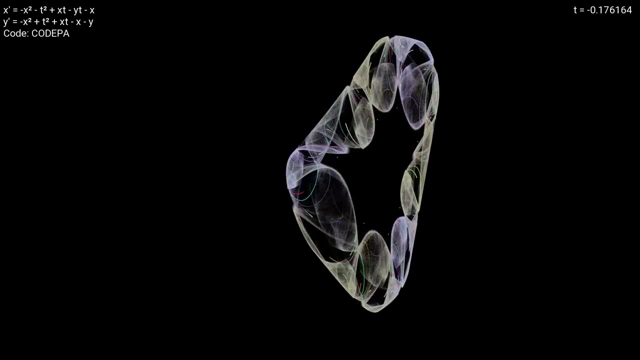 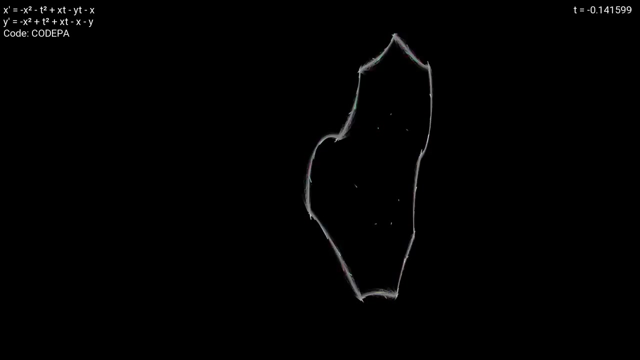